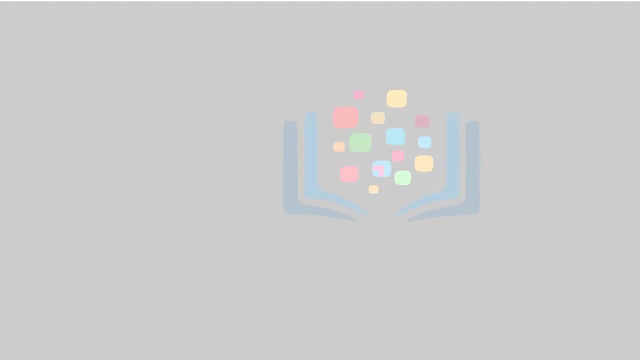 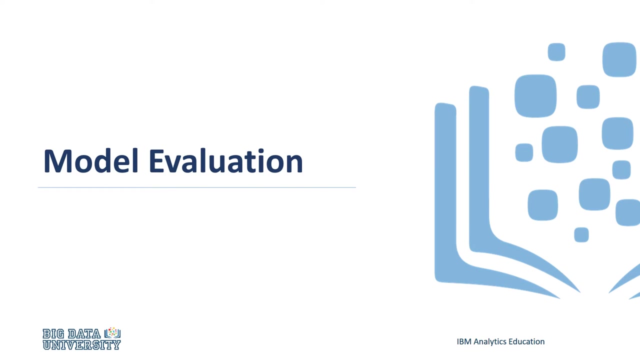 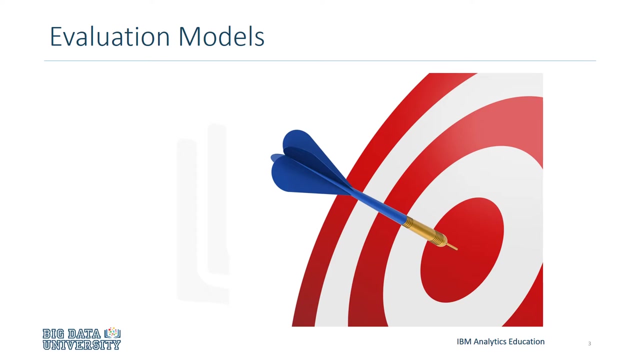 Hello, In this video we'll be covering Model Evaluation. Clearly, when considering evaluation models, we want to choose the one that'll give you the most accurate results, So here we'll introduce and discuss three types of evaluation models that can be used to help with this goal. These models are Train and Test on. 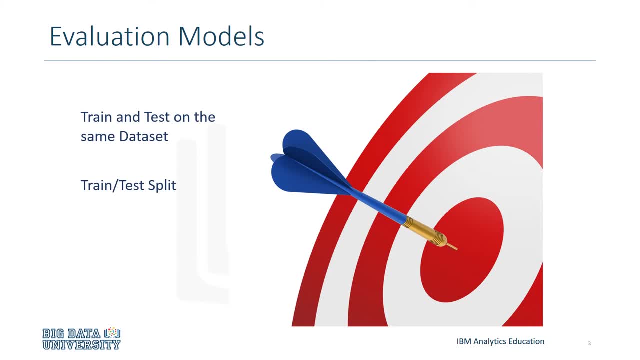 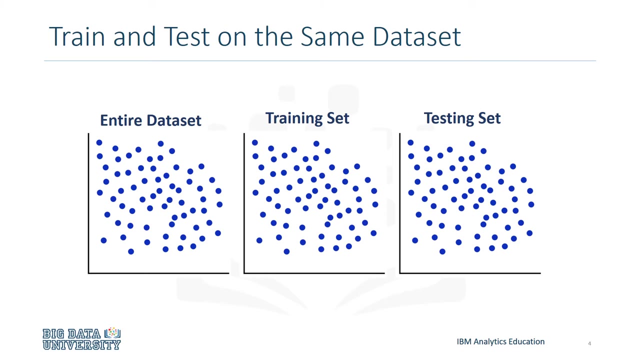 the Same Dataset: Train and Test, Split and Regression Evaluation Metrics. We'll talk about what each of these are, as well as the pros and cons of using each of these models. The first evaluation model we'll talk about is the simplest one: Train and Test on the. 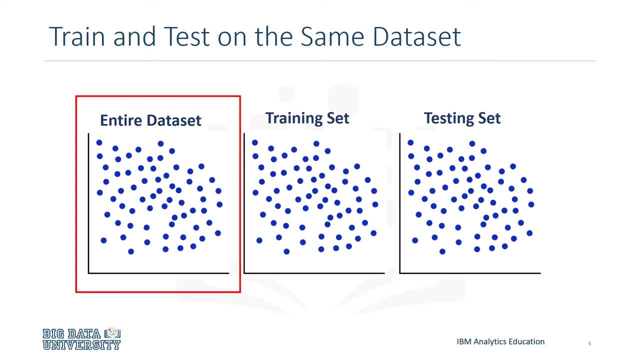 Same Dataset. Essentially, the name of this model says it all. You train the model on the dataset, then you test it using the same dataset. In a general sense, when you test with a dataset in which you know the classification for each data point you're able to obtain. 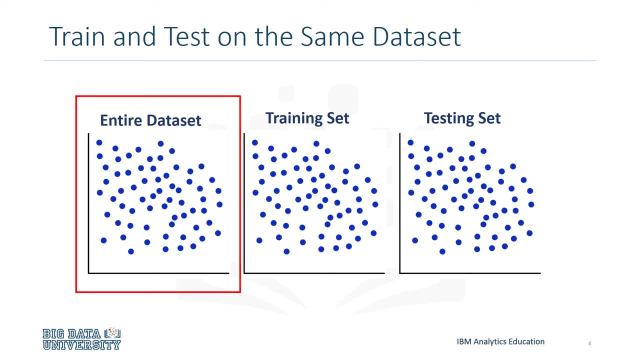 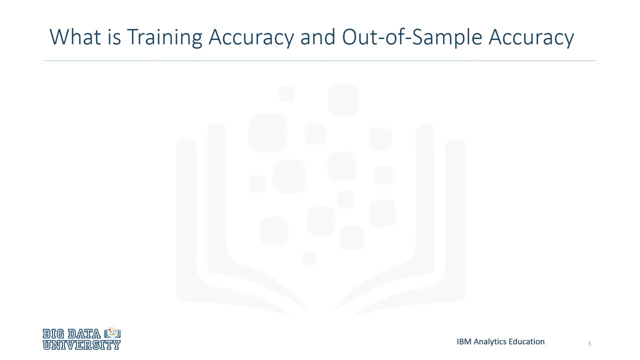 a percentage of accurate predictions for the model. This evaluation model would most likely have a high training accuracy and a low out-of-sample accuracy, since the model knows all the testing data points from the training. We said that training and testing on the same dataset produces a high training accuracy. But what exactly is training accuracy? 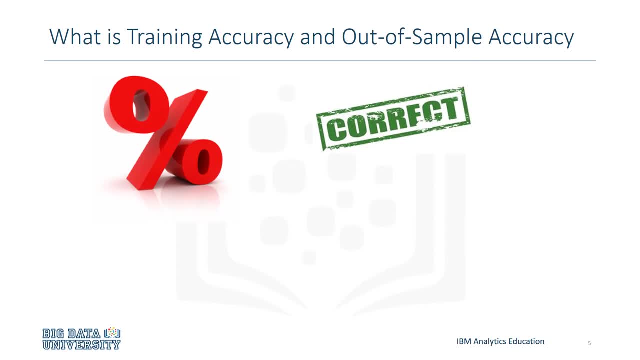 Training accuracy is the percentage of correct predictions that the model makes when using the training dataset. However, a high training accuracy isn't necessarily a good thing. For instance, having a high training accuracy may result in an overfit of the data. This means that the model is overly trained to the dataset, which may capture noise and produce. 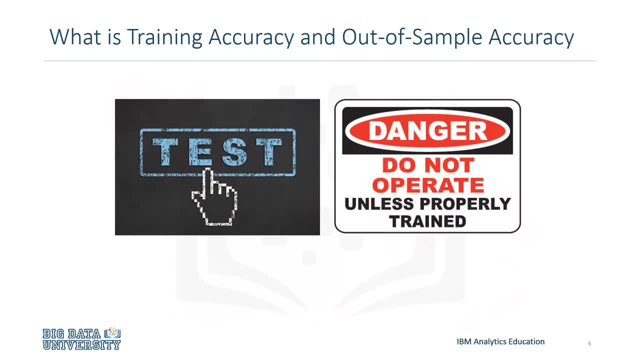 a non-generalized model. Out-of-sample accuracy is the percentage of correct predictions that the model makes on data that the model has not been trained on. Doing train and test on the same dataset will most likely have a low out-of-sample accuracy due to the likelihood of being overfit. It's important that our models have a high 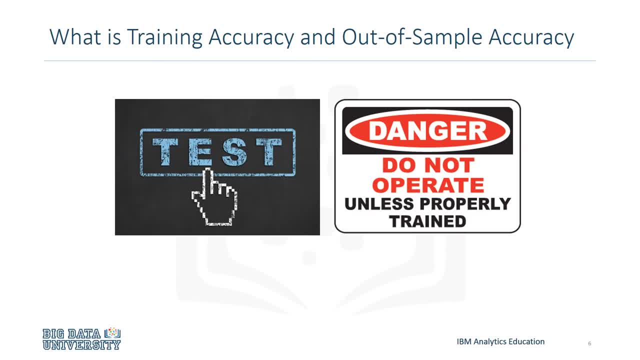 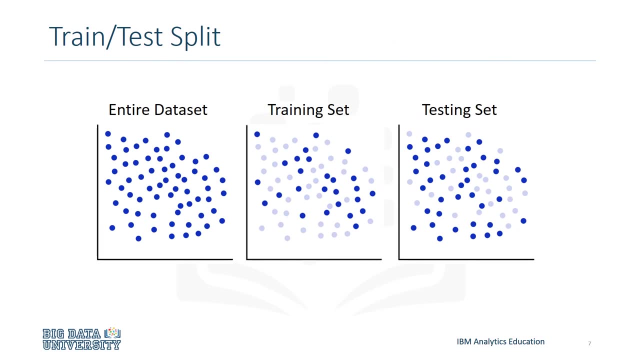 out-of-sample accuracy, because the purpose of any model, of course, is to make correct predictions on unknown data. So how can we improve out-of-sample accuracy? One way is to use another evaluation model. Train-test-split involves splitting the dataset into training and testing sets respectively. 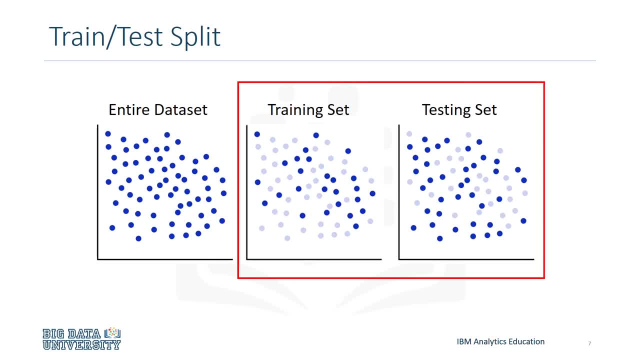 after which you train with the training set and test with the testing set. This will provide a more accurate evaluation on out-of-sample accuracy, because the testing dataset is part of the dataset that could have been used to train the data. This means that we know the 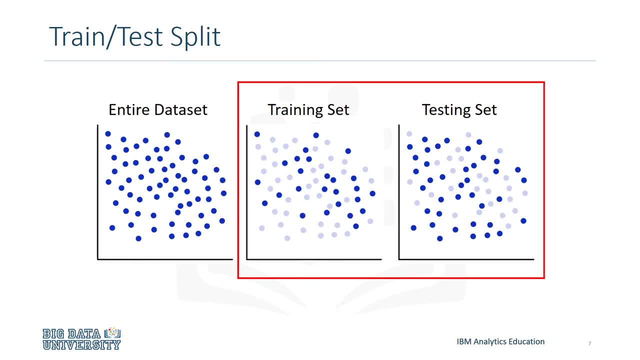 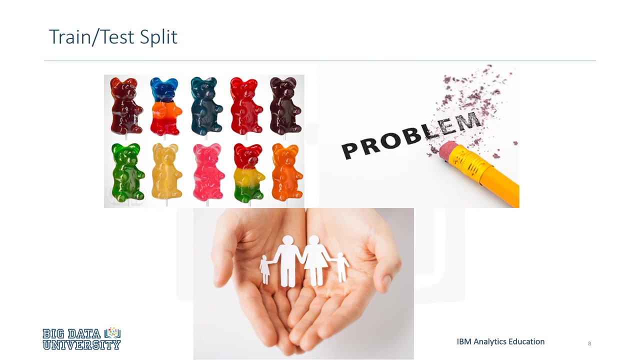 outcome of each data point in the dataset. We have signed off on the use of Run-to-Train mode, which will simply be used to证 In One Exam to evaluate a difference in speed. The whole difference to Run-to-Train mode is important. With this, the model is an alloy. 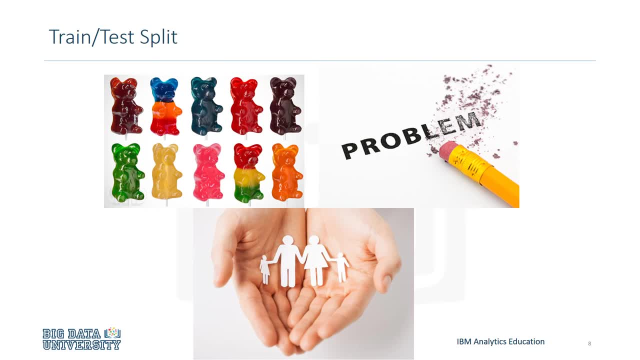 Variation of this causes train-test-split to have a better out-of-sample prediction than training and testing on the same data set, but it still has some problems due to this dependency. Another evaluation model called k-fold cross-validation resolves most of these issues. 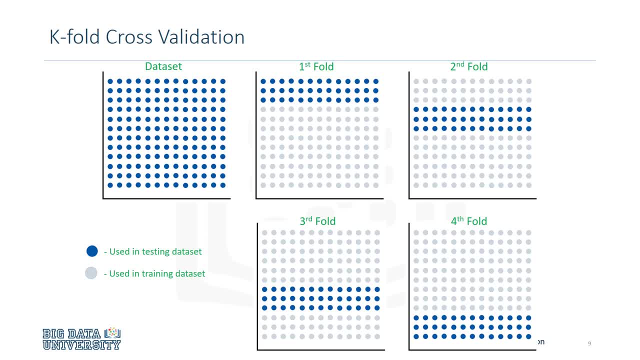 How do you fix a high variation that results from a dependency? Well, you average it K-fold. cross-validation in its simplest form performs multiple train-test-splits using the same data set. where each split is different. Then the result is averaged to produce a more consistent out-of-sample accuracy. 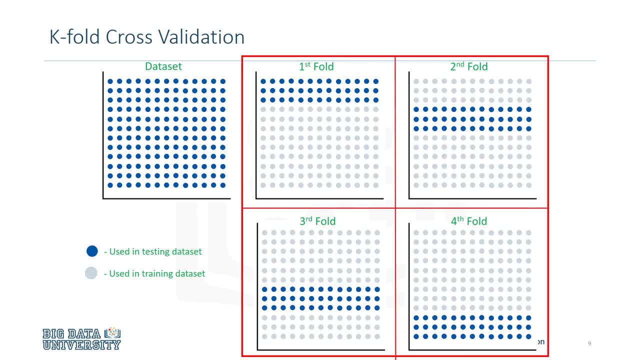 This is better than using a single train-test-split, where our model could test poorly due to a bad train-test-split of the data set, such as having too many outliers in the test set. This example here illustrates the benefits of k-fold cross-validation. 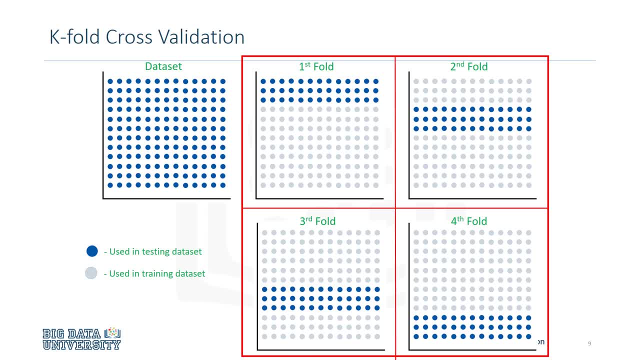 The entire data set is represented by the points in the image at the top left. If we have k equals 4 folds, then one way we can split up this data set is shown here. The results of each fold is then averaged, keeping in mind that each fold is distinct.